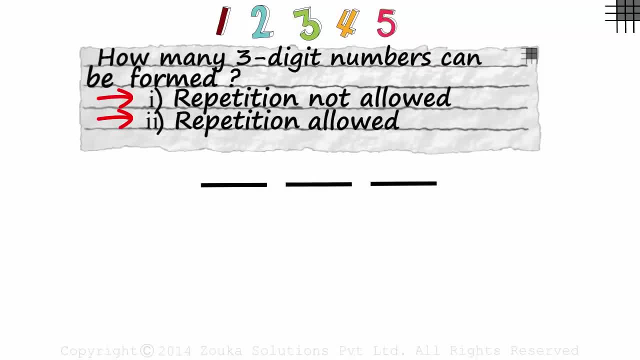 And with this question we have been given two conditions. First, it asks us the answer when repetition is not allowed. Let us understand the first condition: Repetition is not allowed. Look at the number 111.. This is a three-digit number. 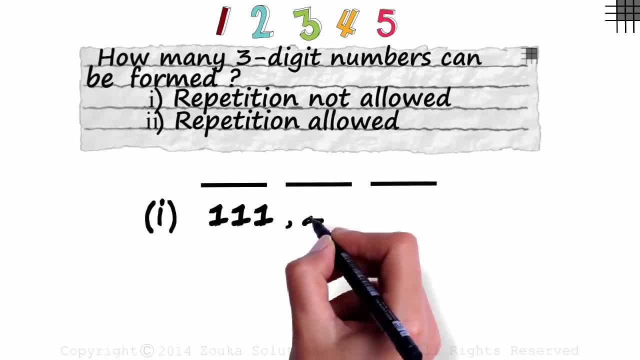 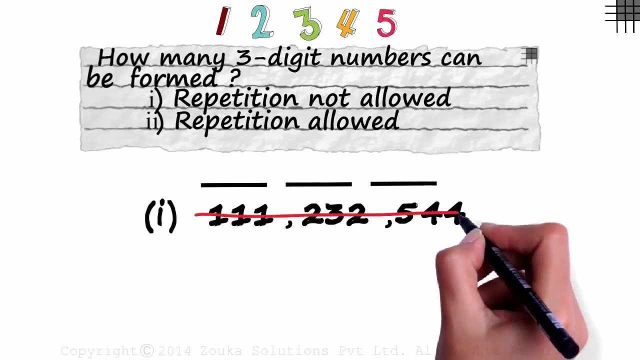 But the digit 1 is repeated. Look at 232 or 544.. The digit 2 is repeated here And the digit 4 is repeated here. By repetition not being allowed, they mean that numbers like these should not be considered. Each of the digits in the slot should be different. 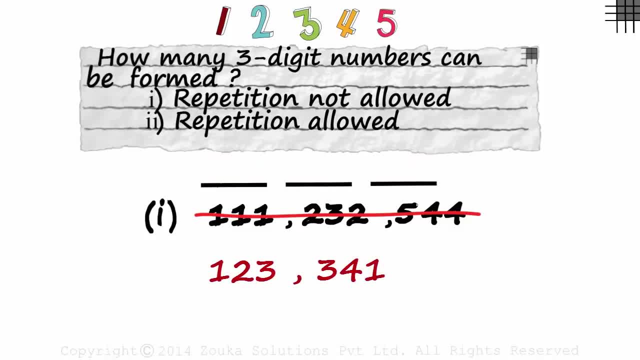 So numbers like 123, 341 or 524 are allowed as the digits in each case. The digits in each case are different from each other, So let's make three slots for the digits again. Now you can start thinking How many three-digit numbers can be formed if repetition is not allowed. 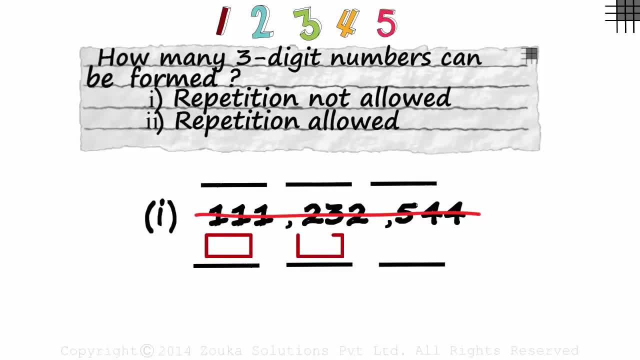 Before you think of the three-digit numbers, look at the slots individually. Let's look at the first slot, or the hundreds place. In how many ways can you fill the first slot? It is a simple question. You don't need to know permutations. 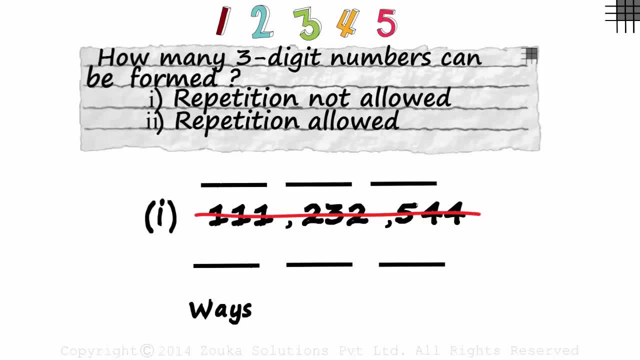 You don't need to know permutations or combinations for this. In how many ways can you fill the first slot? You can fill it with any of the five digits, right. You can fill it with a 1 or a 2 or a 3 or a 4 or a 5.. 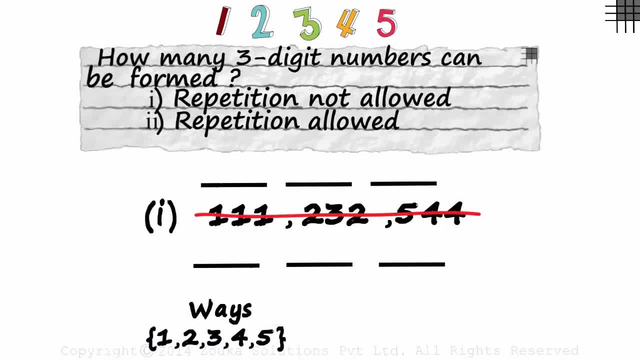 These are the five digits given to us. Did you listen carefully? I used the word OR One, or a two, or a three, and so on, So five ways in all. We can fill it with any one of these five digits. We can fill it with any one of these five digits. 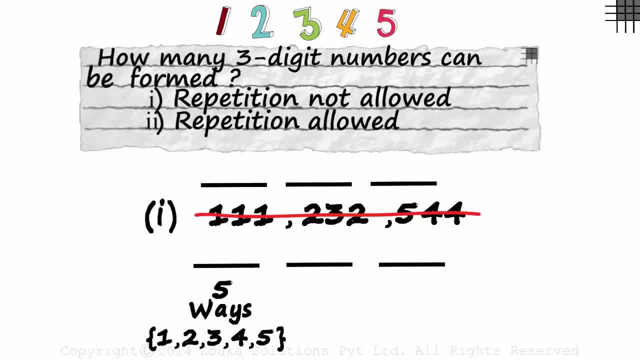 Okay, now listen to the next question carefully. Having filled this slot with one of the digits, in how many ways can we fill the second slot? Easy, We have used one of the digits here. It can be any digit, doesn't matter. 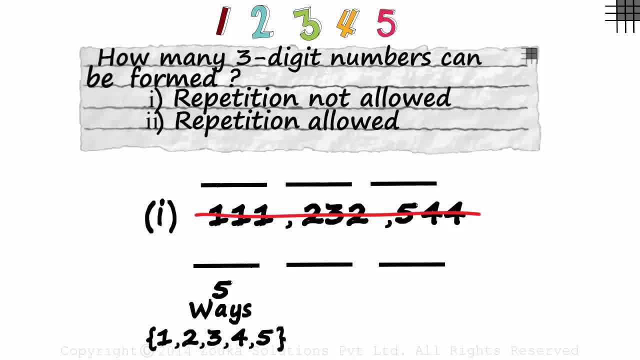 But after having used one, four digits remain. So the second slot can be filled in four ways. If we fill the first slot with one, we have two, three, four, five, six, seven, eight, nine, ten, eleven, twelve, thirteen, fourteen, seventeen, eighteen, nineteen, nineteen, twenty. 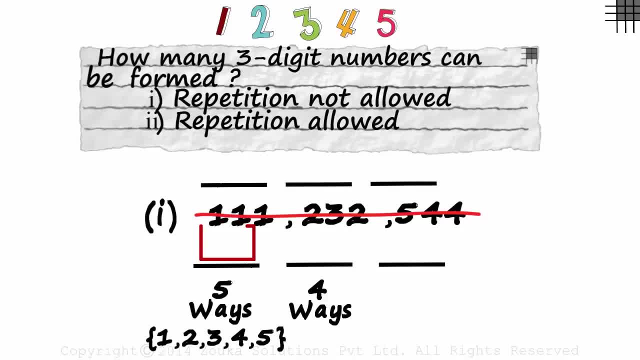 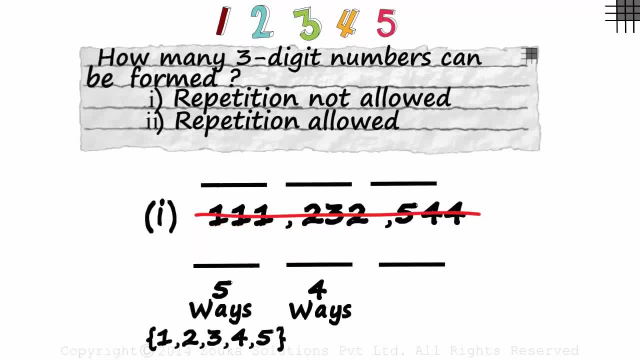 for the second slot. Now tell me, Having filled the first and the second slot, In how many ways can the third slot be filled? It's simple: We have used up two digits here. Only three remain. The third slot can be filled in three ways. 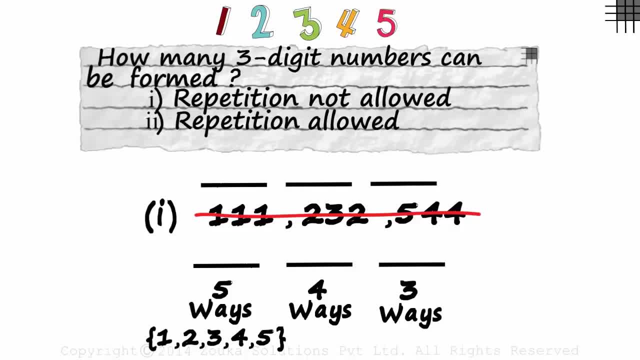 We're almost done Almost. The first slot can be filled in five ways, the second in four ways and the third in three ways. So how many three-digit numbers can be formed if repetition is not allowed? Do we add these three or do we multiply them? 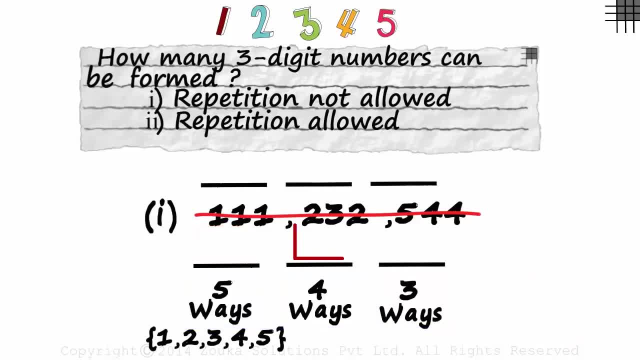 What are we doing? Are we filling in the first slot or the second slot or the third slot, Or are we filling in the first slot and the second slot and the third slot? It will be, AND, Yes, we are filling all three slots and not just one. 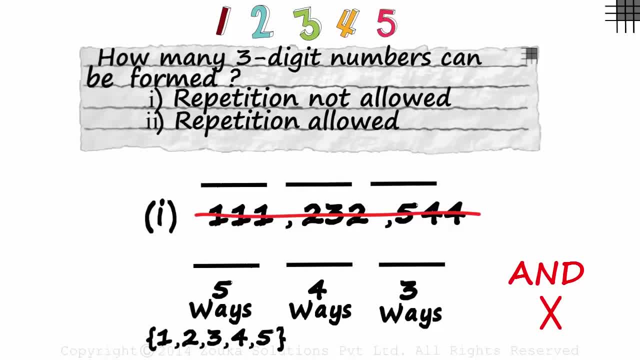 AND, as we have seen in the previous session, is multiplication. So we multiply these three: 5 times 4 is 20 and 20 times 3 is 60. There are 60 ways in which we can form three-digit numbers. 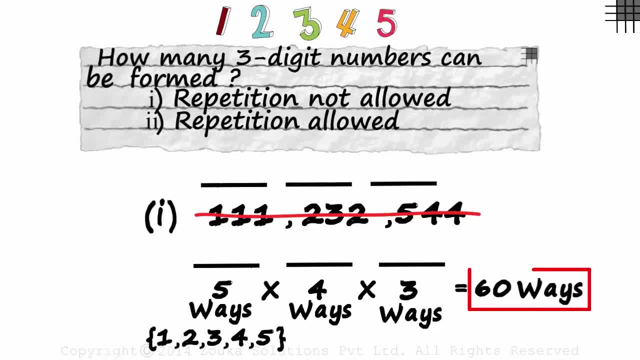 without repetition of four. We can also form three-digit numbers without repetition of five digits. These include numbers like 123, 314, 245 and so on. No repetition. Hope this was clear. Here we started off with the hundreds place. 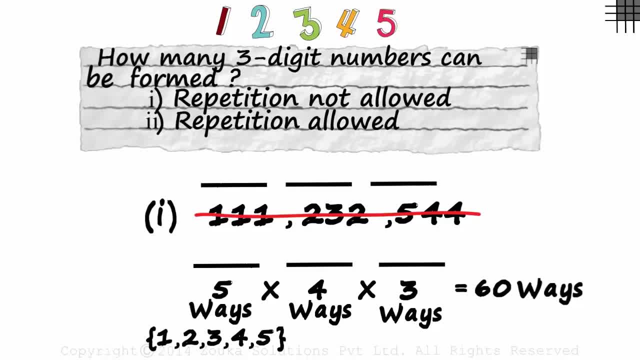 Can we start off with the units place? Of course, yes, we could have. If we would have started off with the units place, we could say that the units place could be filled in five ways. If the units place is filled, the tens place would be filled with any of the remaining four digits. 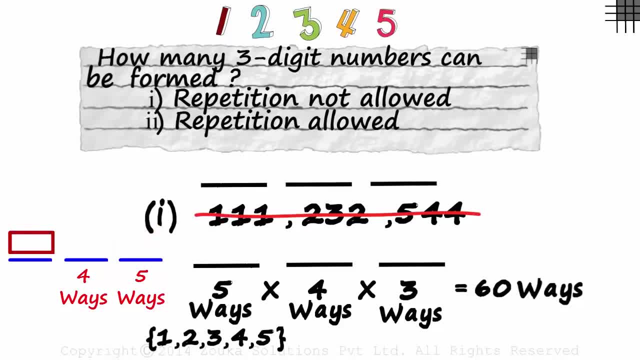 And once two digits are utilized, the hundreds place can be filled with any one of the remaining three digits. Three times four times five will also give us the same answer 60 ways. If you really understood this, then understanding the second stated condition would be super easy. 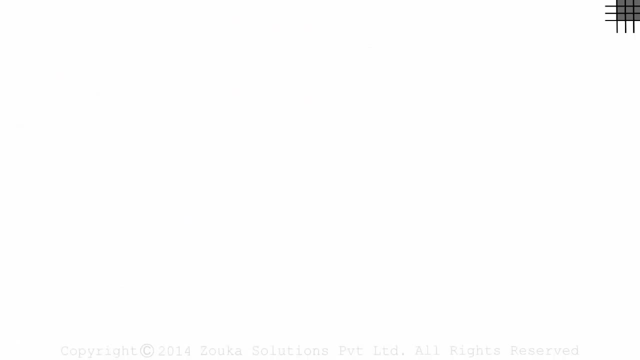 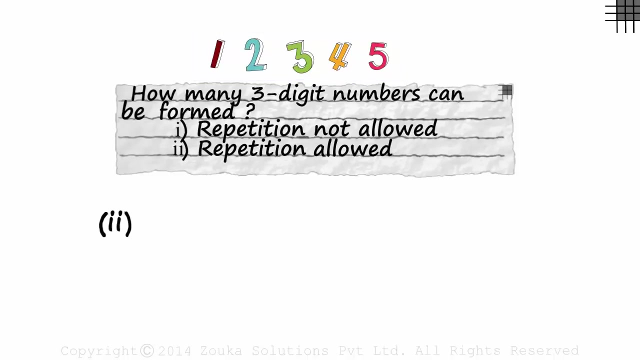 Let's repeat the question on a new page. This time we solve the question keeping in mind the second condition: Given these five digits, how many three-digit numbers can be formed, assuming repetition is allowed? So now we are allowed to consider numbers like 111 or 322, and so on. 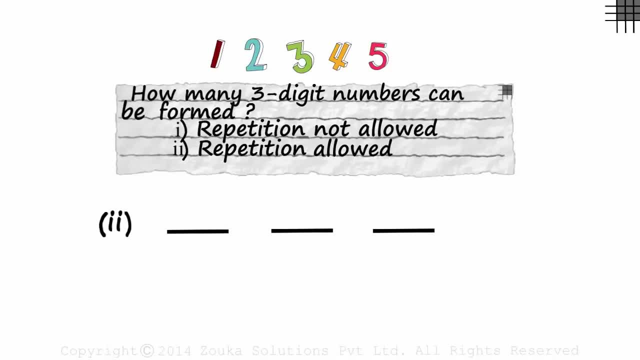 So we have three slots for the three digits. How many three-digit numbers can be formed when repetitions are allowed? I want you to try this. Remember, repetitions are allowed. So now we are allowed to consider all numbers which we had ignored earlier. 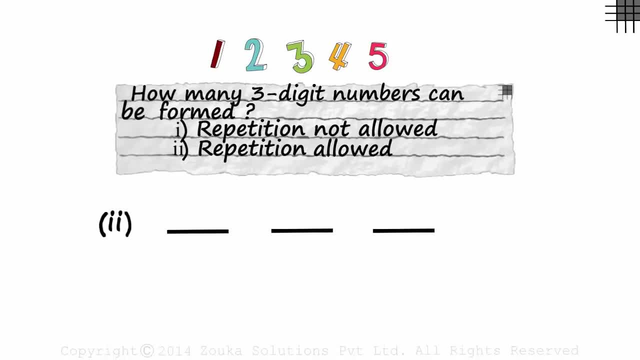 We should have the possible numbers greater than 60.. Try it. Okay, as we saw earlier, let's go slot by slot. In how many ways can the hundreds place be filled? It can be filled with any one of the five digits we have. 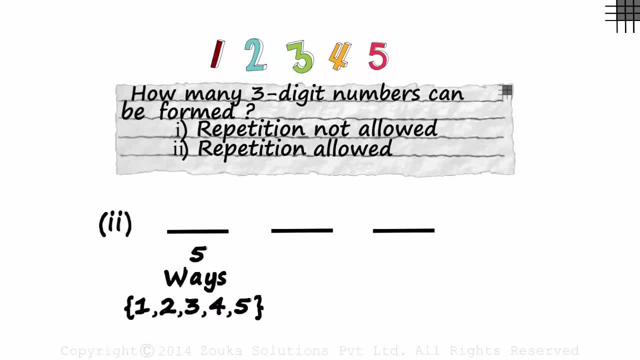 It can be filled in five ways. Now, in how many ways can the second slot be filled? Think well, The second slot can also be filled in five ways. Why? It's because repetitions are allowed. If we used up one digit here, the same one can be used here as well. 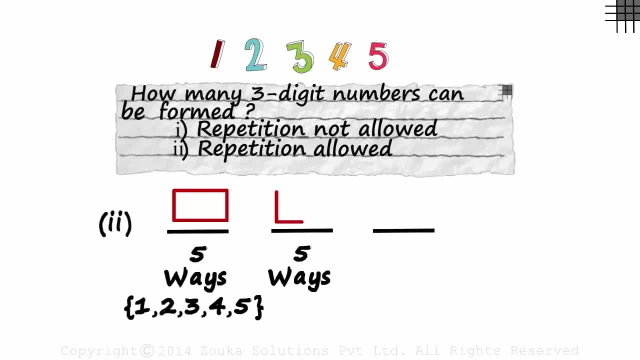 So no matter what digit is used in the hundreds place, the tens place can be filled with any one of the five digits, And similarly the third slot can also be filled with any one of the five digits. Five ways again, If we have one in the hundreds place. 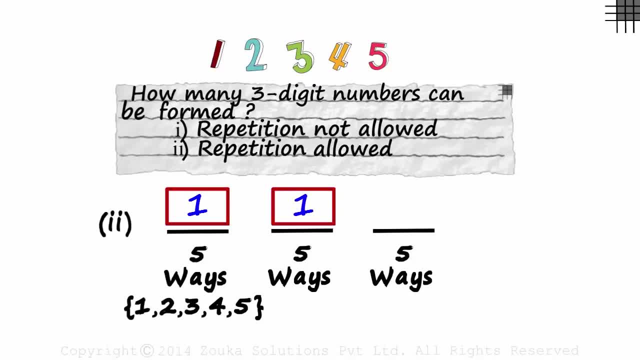 the same one can be used in the tens place and in the units place as well. There are no restrictions here. So as we are filling in the first and the second and the third slot, we multiply these three numbers and get the answer as one hundred and twenty five.